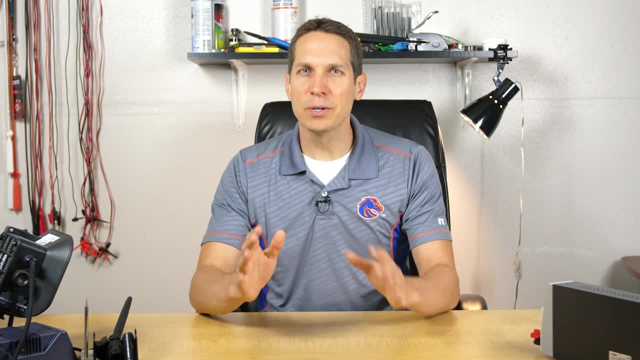 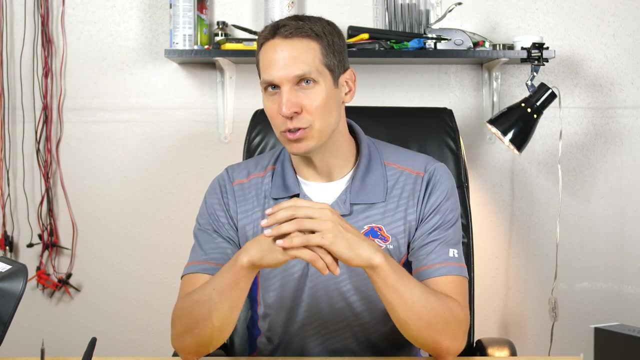 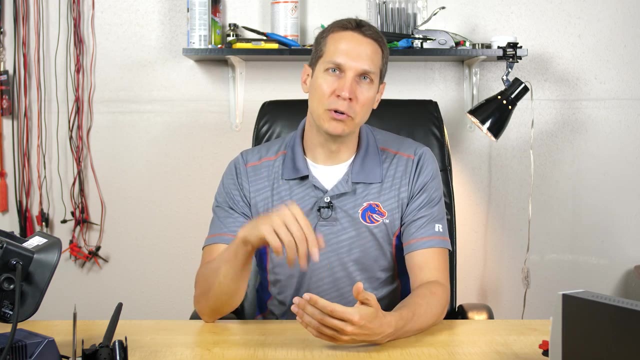 Today we're going to discuss the basics of semiconductors and their role in the field of electronics. Before semiconductor devices existed, vacuum tubes were the only devices available for signal amplification, switching and other applications. Though vacuum tubes are functional, they are bulky, require a high operating voltage and are pretty inefficient. 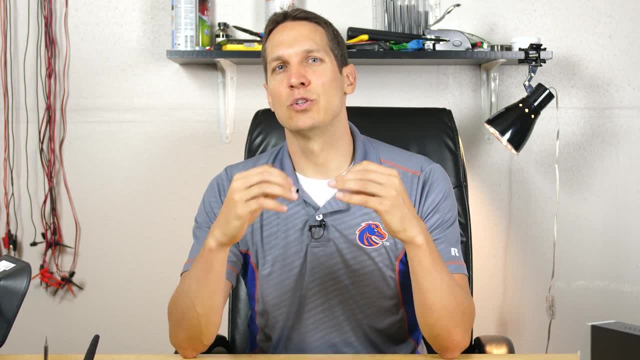 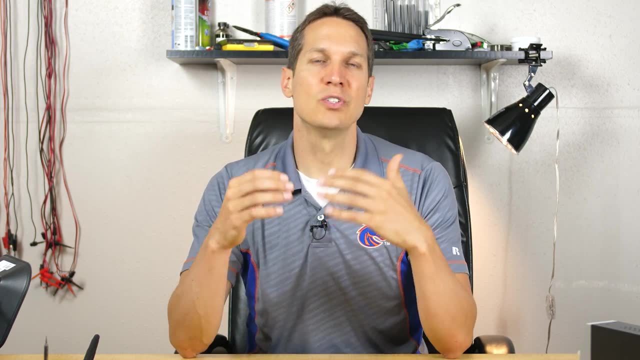 When semiconductor devices like transistors were invented, semiconductors started to acquire a dominating role in electronics. Semiconductors are materials that are in between conductors and insulators when it comes to the ability to conduct electrical current, which explains the name The most commonly. 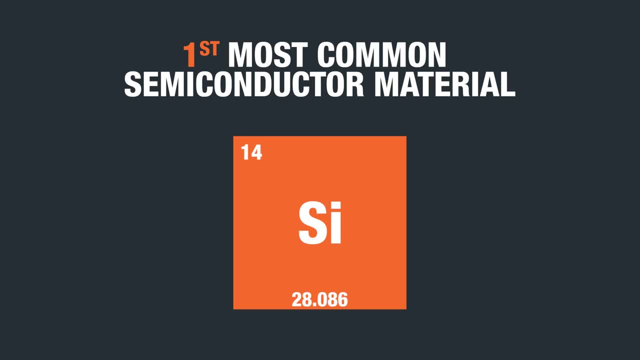 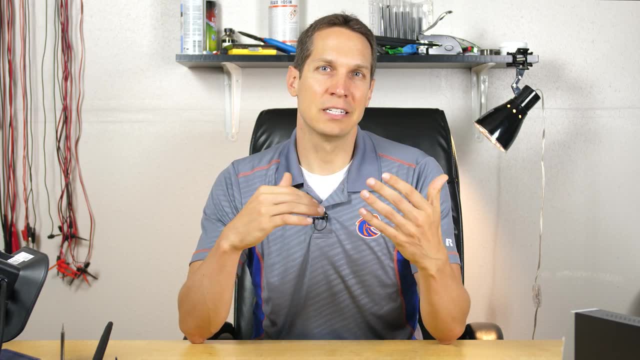 used semiconductor material in the electronics industry is silicon. After that it is a compound known as gallium arsenide. Though germanium was used extensively in the early years of semiconductor technology, it is unstable at high temperatures, so silicon became much more widely used. 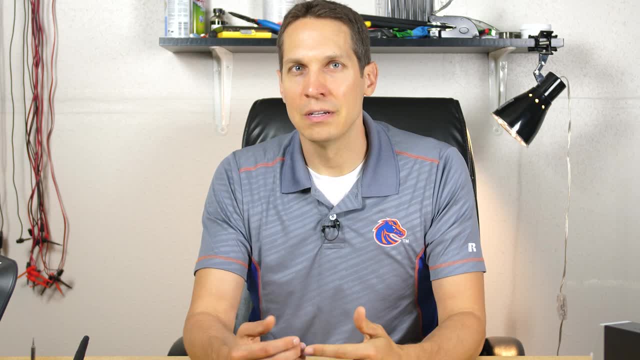 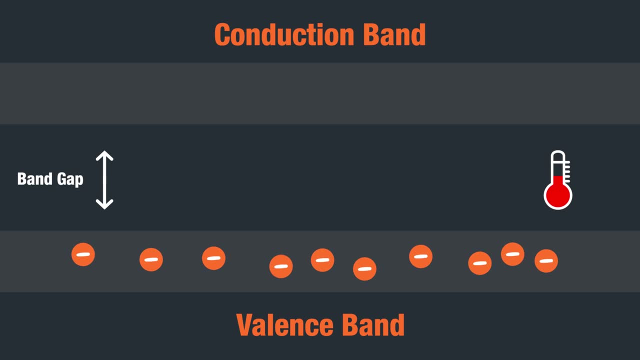 Semiconductor materials have two current carriers: free electrons and holes In an intrinsic semiconductor material. free electrons are produced when the material receives a current current. Free electrons are produced when the material receives sufficient thermal energy that provides valence electrons from the valence band- enough energy to jump to. 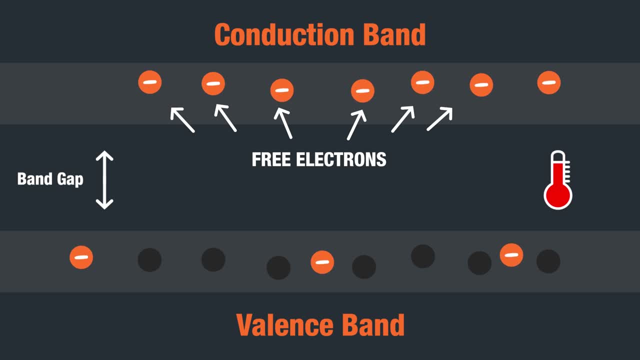 the conduction band and turn into free electrons. When valence electrons jump to the conduction band, they leave vacancies in the valence band. These vacancies are called holes. The number of holes in the valence band is just equal to the number of free electrons in the 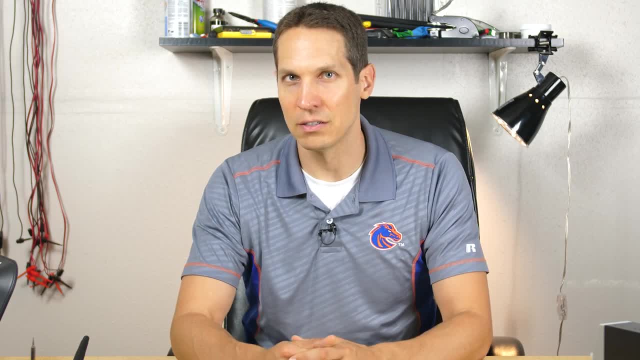 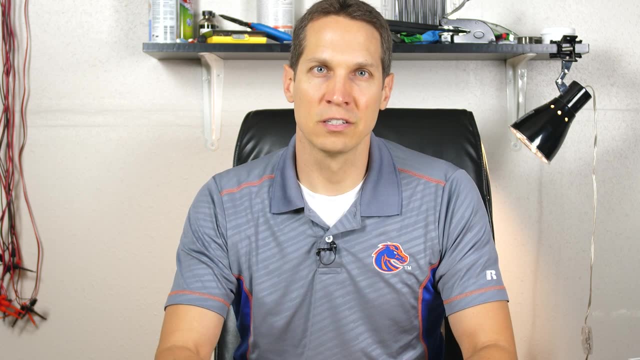 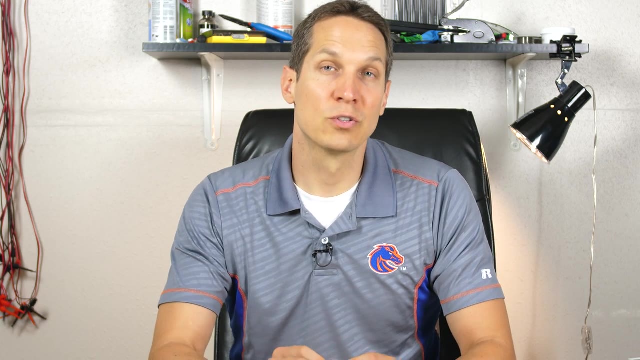 conduction band in this undoped intrinsic material. A semiconductor material becomes a useful electronic component by controlling its conductivity. However, semiconductor materials in their intrinsic state do not conduct current well. This is because of the limited number of free electrons and holes in it. but through a process known as doping, the conductivity. 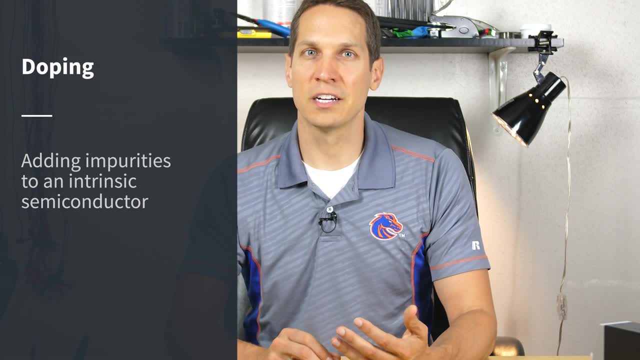 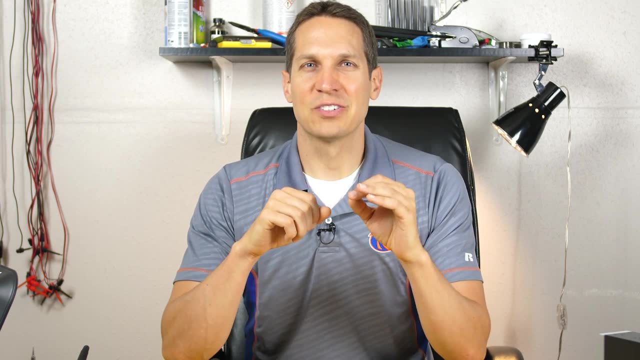 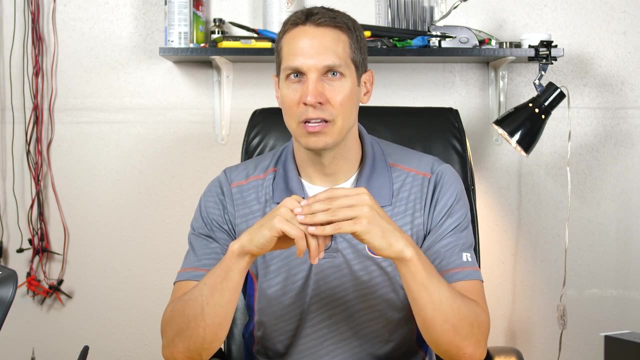 of a semiconductor can be increased. Doping increases the number of current carriers by adding impurities with either more free electrons or holes to the intrinsic semiconductor material. The number of free electrons in an intrinsic semiconductor material with four valence electrons, such as silicon, is increased in the doping process by adding pentavalent impurity atoms. or atoms with five valence electrons, such as arsenic, phosphorus, bismuth or antimony. To visualize this, let's examine a phosphorus atom covalently bonded with four adjacent silicon atoms. As we can see, only four valence electrons of the phosphorus atom are used. 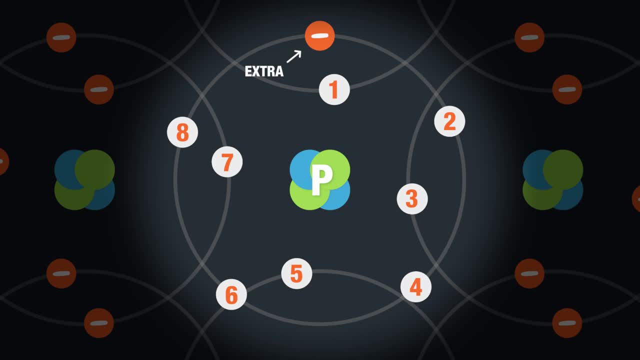 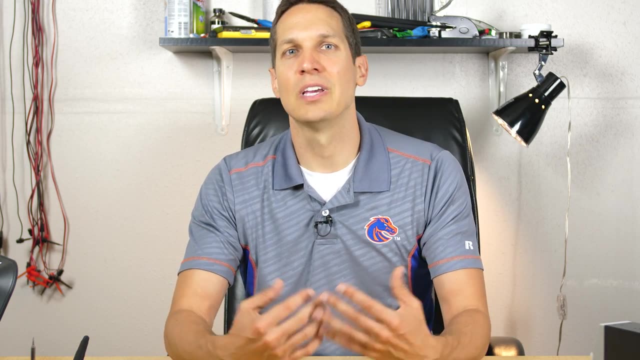 to form covalent bonds with the silicon atoms, leaving an extra electron. At lower temperatures that extra electron stays with the impurity or donor atom, but when the temperature increases it becomes a free electron. Once the electron has moved into the conduction band, the doping, 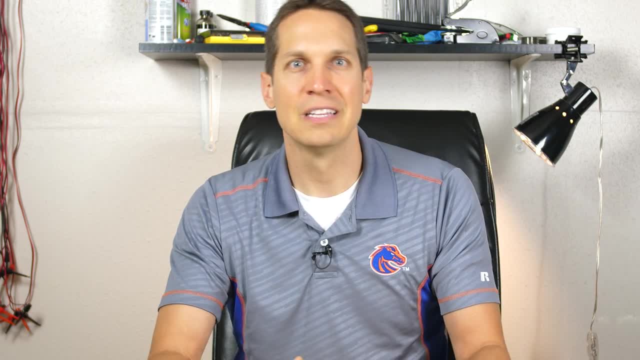 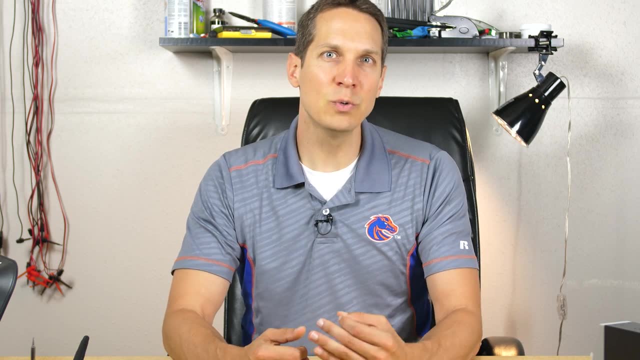 atom is now positively charged, as there are more protons in the nucleus than electrons in orbit. Finally, while the electron is free to move about, the atom itself is fixed in place and will not move, even with an applied voltage across the material. So by adding 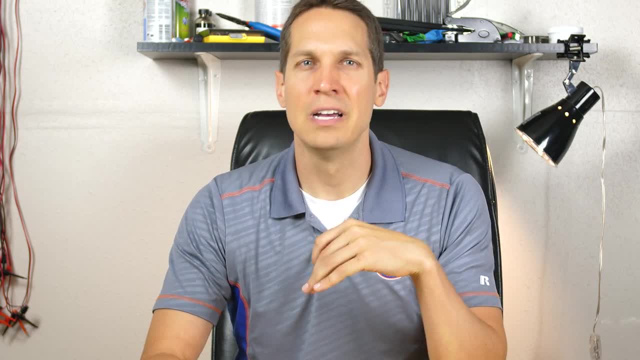 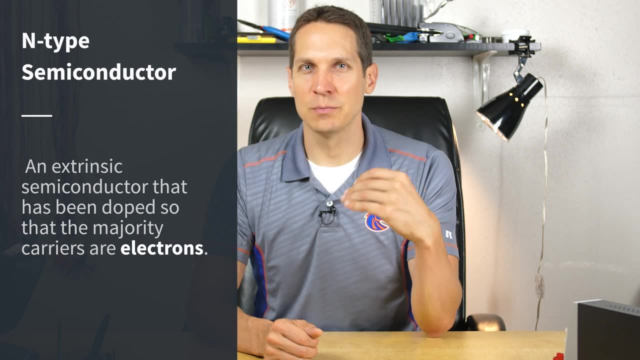 pentavalent impurity atoms to an intrinsic semiconductor material, the number of free electrons can be increased, as well as the conductivity of the semiconductor material. Semiconductors doped with pentavalent atoms are n-type semiconductors, since the majority 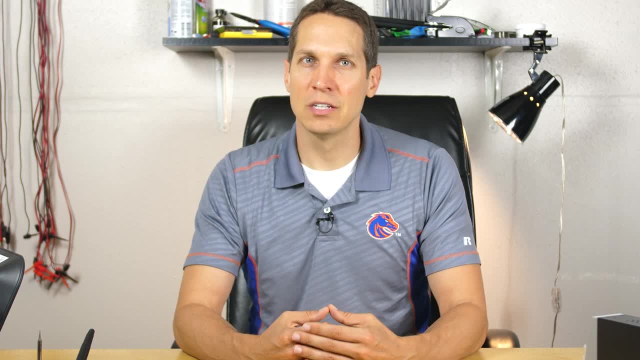 of its current carriers are electrons. In order to form a free electron, the semiconductor is now positively charged. as there are more electrons in the nucleus than electrons in semiconductor material with four valence electrons, such as silicon, to have more holes, they 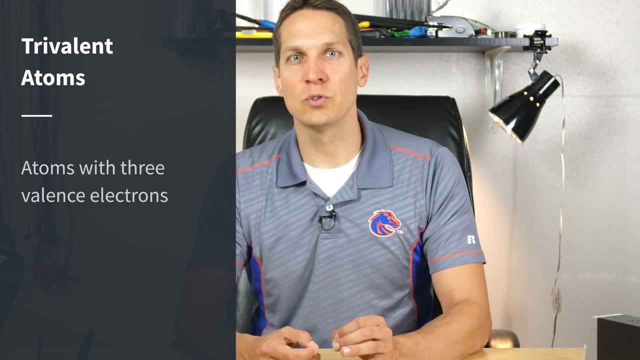 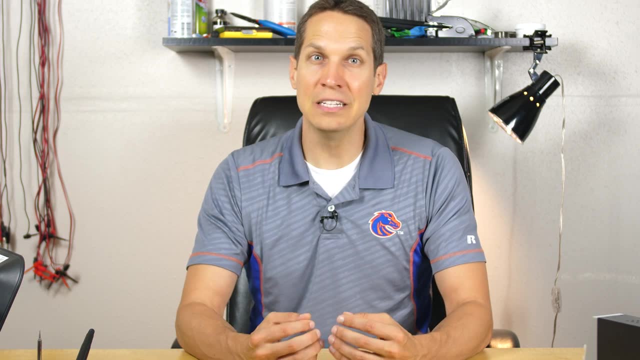 are doped with trivalent impurity atoms. These are atoms with three valence electrons in their valence shell, like boron, indium and gallium. To understand how trivalent impurity atoms increase the number of holes in an intrinsic semiconductor material, let's see a boron. 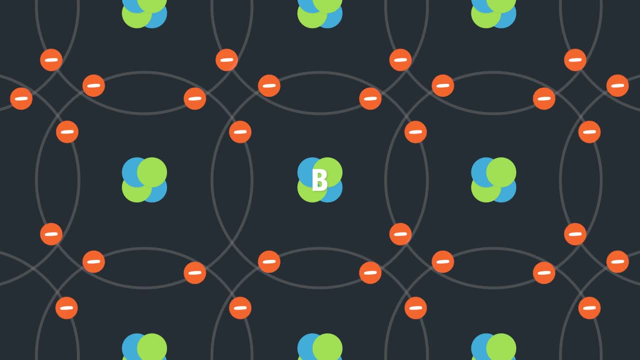 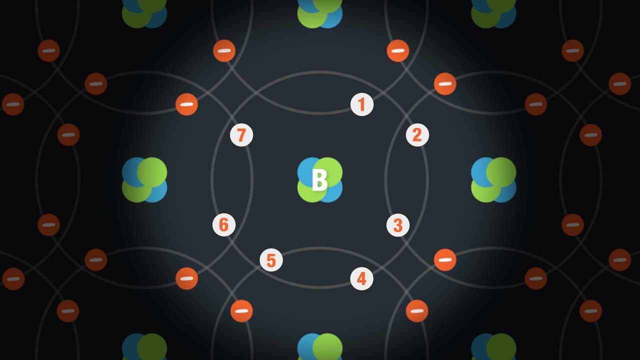 atom attempt to form a covalent bond with the four adjacent silicon atoms. In this case, at lower temperatures, when the boron covalently bonds with its neighbors, the fourth silicon atom doesn't make a bond. As the temperature increases, an adjacent silicon atom donates. 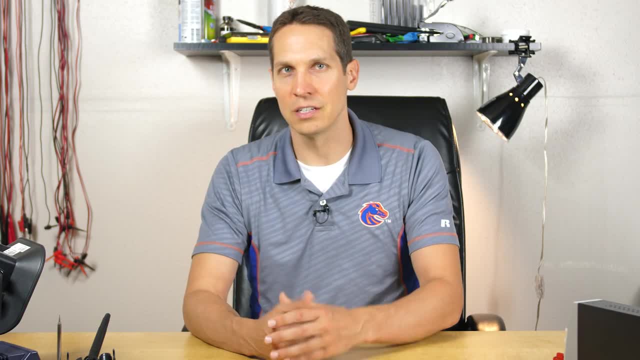 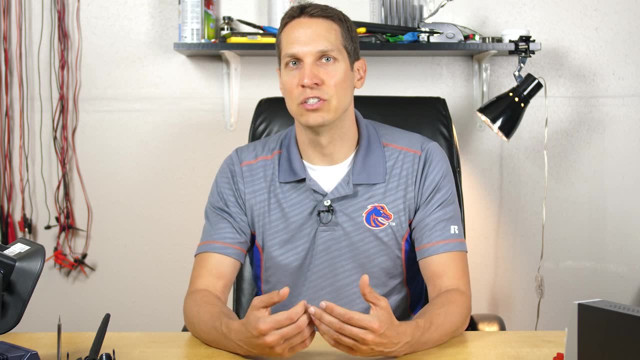 an electron to complete the fourth bond between the boron and silicon atoms. There is now a hole where the adjacent silicon atom gave up its electron and the boron atom is negatively charged as it has an additional electron. In this case we can say that by adding more. trivalent impurity atoms to an intrinsic semiconductor material. it increases the number of holes and improves the conductivity of the semiconductor material. Semiconductors doped with trivalent atoms are are first of all p-type semiconductors, since the majority of its current carriers are holes. 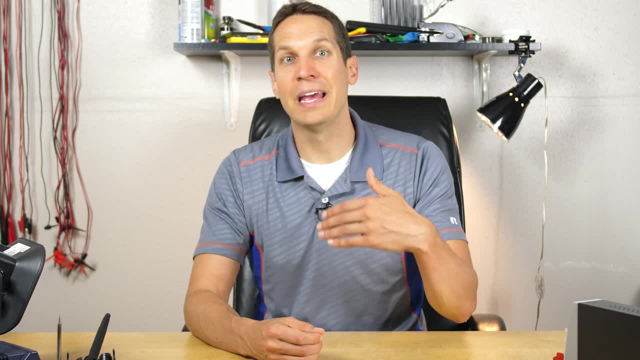 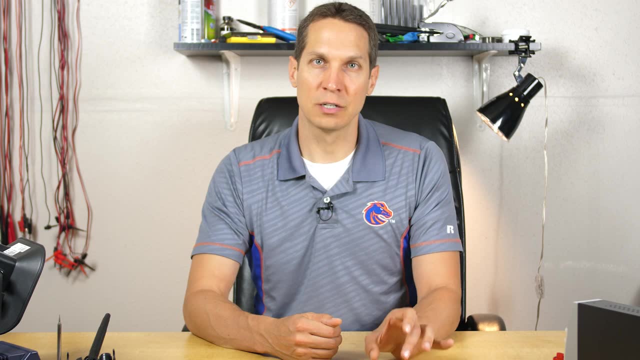 The doping process converts an intrinsic semiconductor material into an extrinsic and produces either an n-type or p-type semiconductor material. When you dope an intrinsic semiconductor p-type and then directly adjacent to that n-type, the boundary where the p-type and n-type doped, 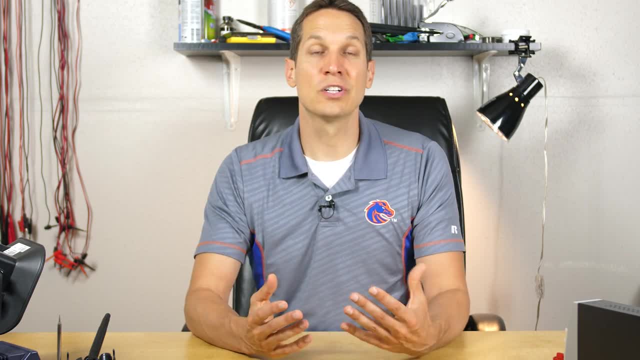 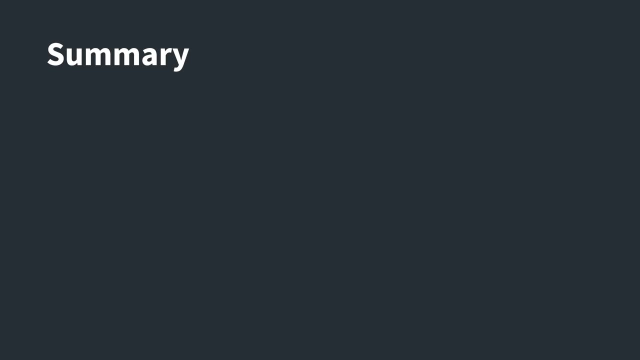 material touches is known as a p-n junction. This p-n junction is the basis for different semiconductor devices widely used today, like diodes, transistors and thyristors. So in this video we talked about the basics of semiconductors: the intrinsic semiconductor. 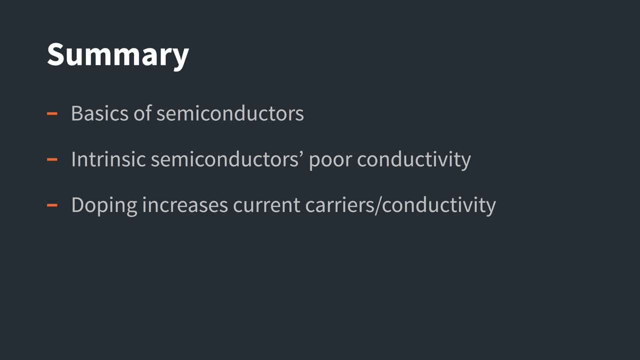 and its poor conductivity. how doping increases the number of current carriers in a semiconductor material and improves its conductivity. We also briefly mentioned how different semiconductor devices were created based on the p-n junction. If you have any questions, leave it in the comments below, and if you found this interesting or helpful, please subscribe to our channel. and like this video.